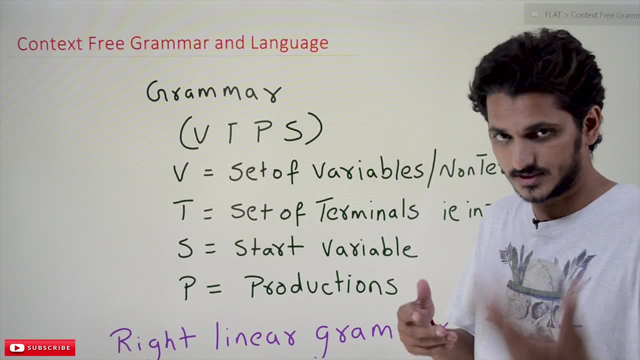 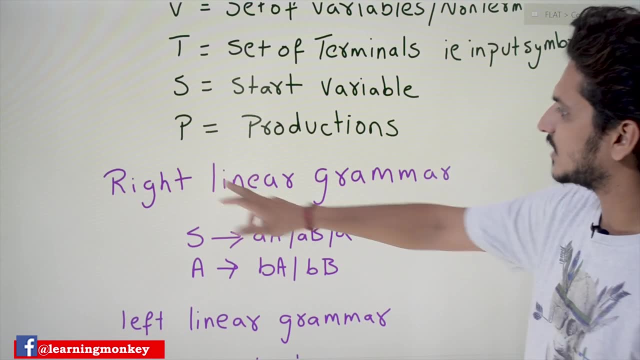 that will, that productions will go, will generate the strings that are present in our language. Based on that, we have to write the productions. In our previous classes, when we discussed about right linear grammar, S tends to AA or AB or A. This is how. 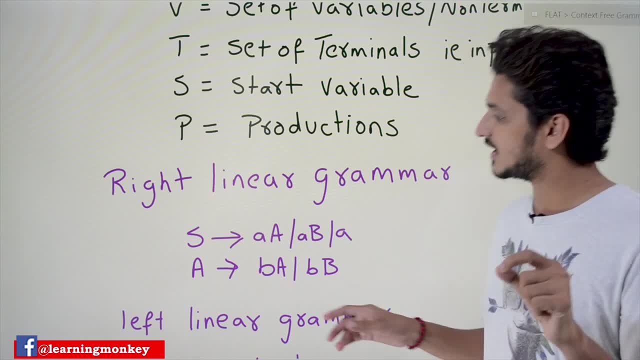 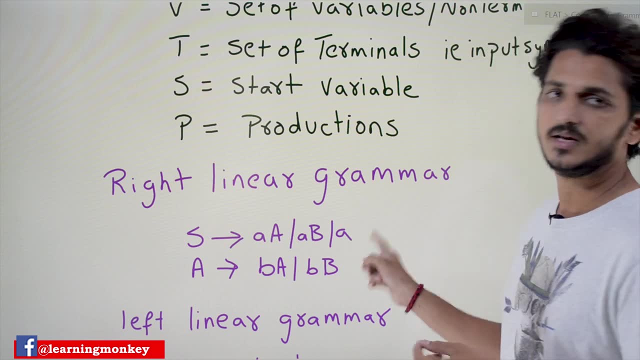 the productions will be. What's the conditions for right linear grammar? Left side should have a non-terminal and right side you should have a terminal, followed by non-terminal or terminal. These are the conditions for productions. You should not avoid that. conditions Based on that. 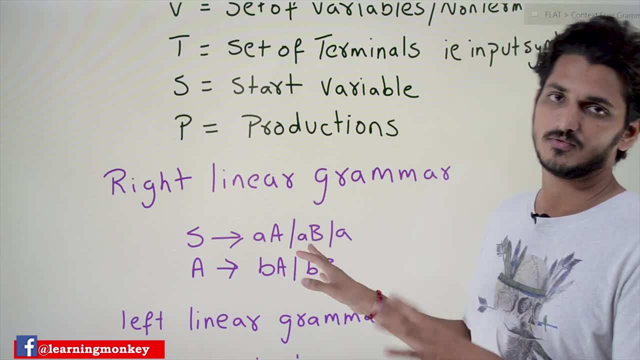 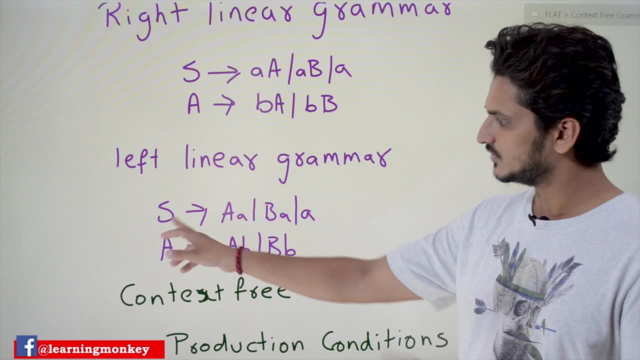 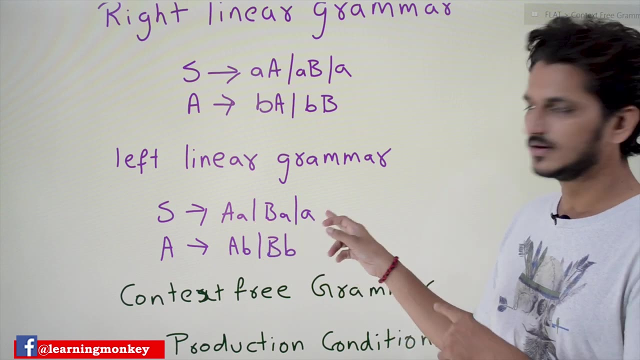 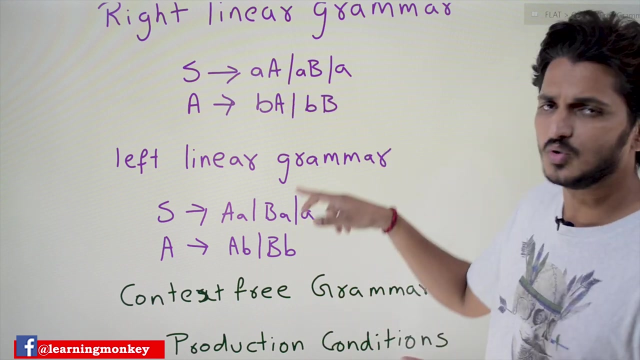 conditions: only you have to write the right linear grammar. Productions for right linear grammar. Similarly, what's the left linear grammar is left side. Left side you can have a single non-terminal. On the right side you can have a non-terminal followed by a terminal or single terminal. These are the conditions for productions of left linear grammar. So all this grammar is used to identify, to write the grammar for regular languages. 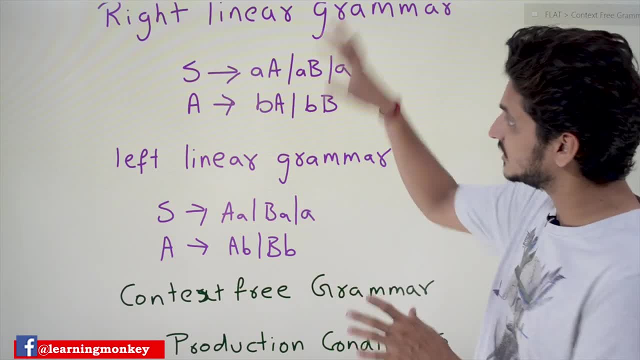 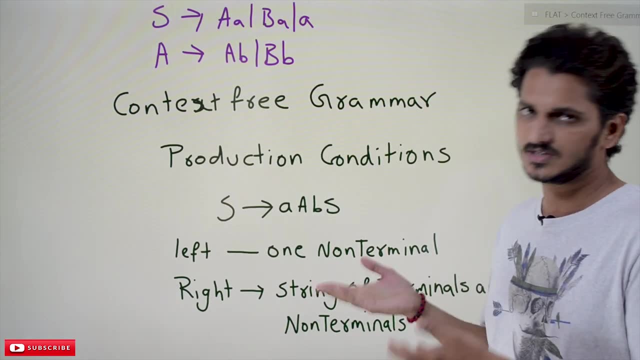 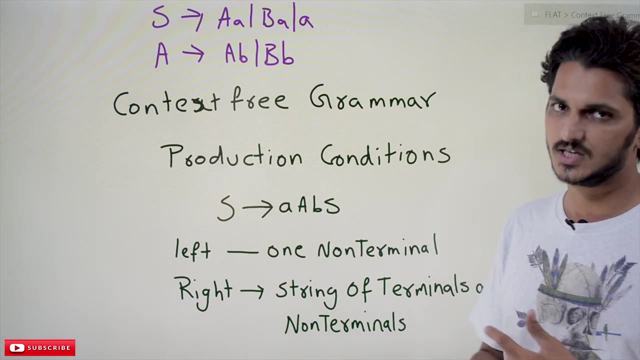 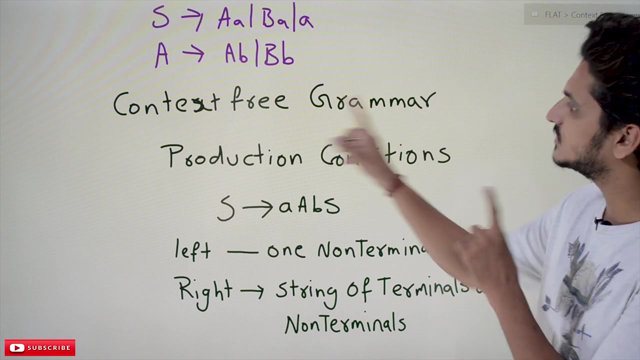 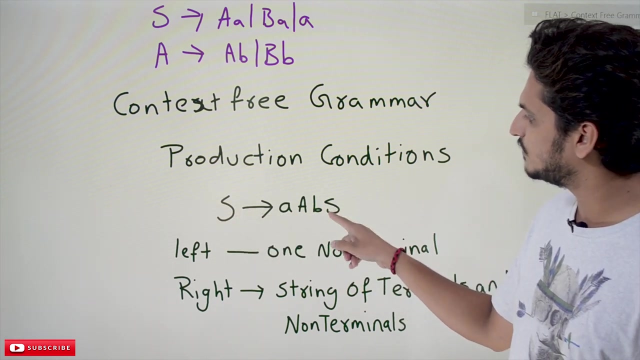 Okay, this is how. this is what we have discussed in our previous classes up to here. Now, coming to the context-free grammar. Similarly we are having in this grammar also we are having same productions: VT, PS, V means set of non-terminals, T means set of terminals, S means starting symbol, where we have to start the grammar, And next the production conditions. In the context-free grammar we are having set of conditions to write the productions. What's those productions? S tends to A capital, A B small capital, S Here capitals means 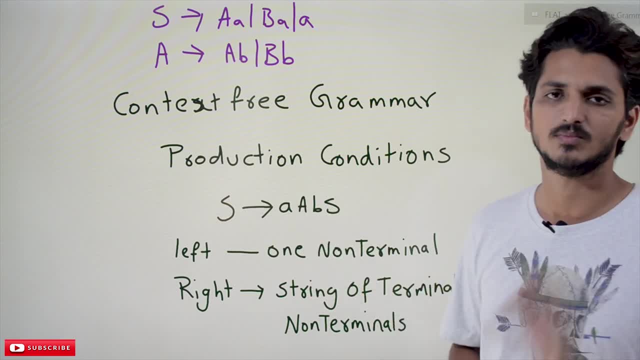 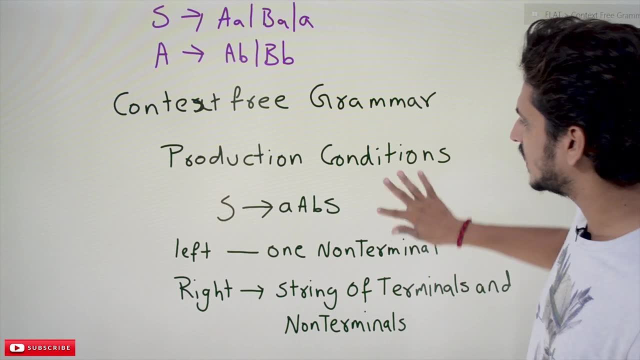 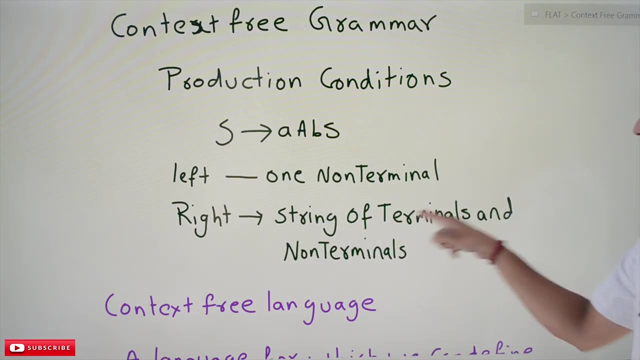 these are non-terminals. Small letters means those are terminals. Okay, we have to follow this conditions. What's this condition? On the left hand side, you should have one non-terminal. On the right hand side, you can have a string of terminals and non-terminals. On the right hand side, you can have string of terminals and non-terminals. 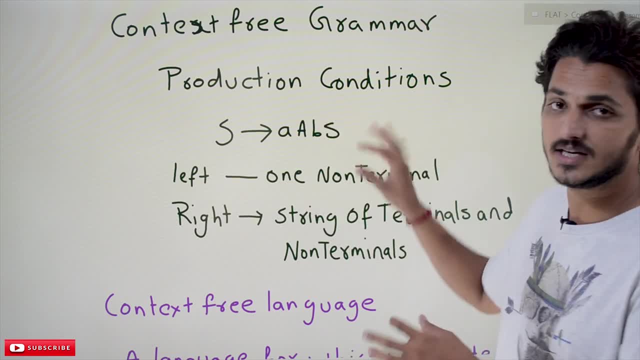 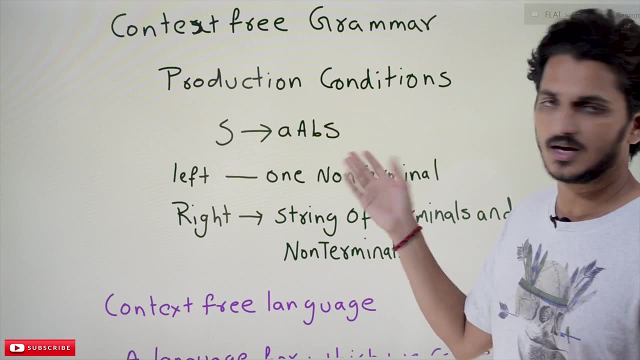 You can write it any way On the right hand side. there are no conditions. You can write any situation String of A, A, B, B, like that, b a, s, any how you can write. you can have a string of a terminals and non-terminals. this is the. 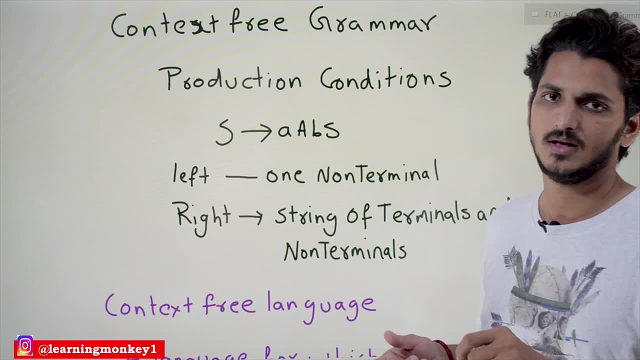 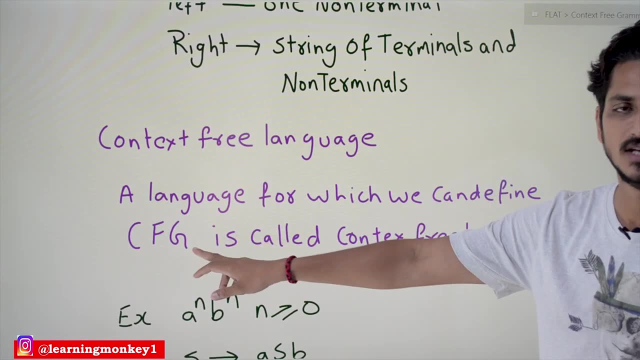 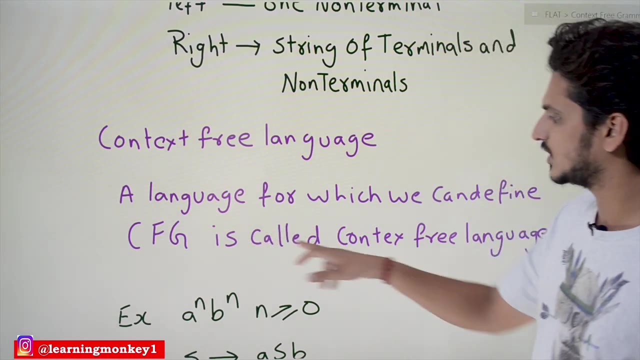 condition to write the productions for context-free grammar. okay, then what's context-free language? a language for which we can define c of g for a language, if you define context-free grammar, then we say it as context-free language and that language we call it as context-free language. 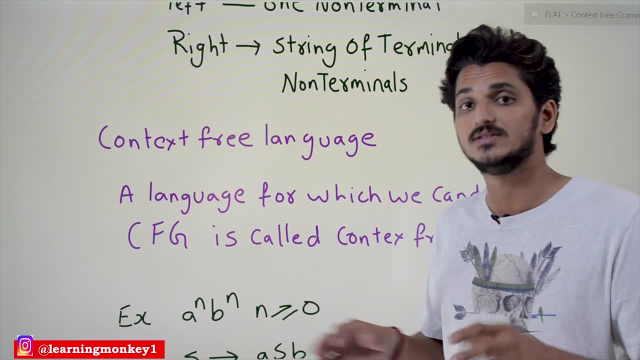 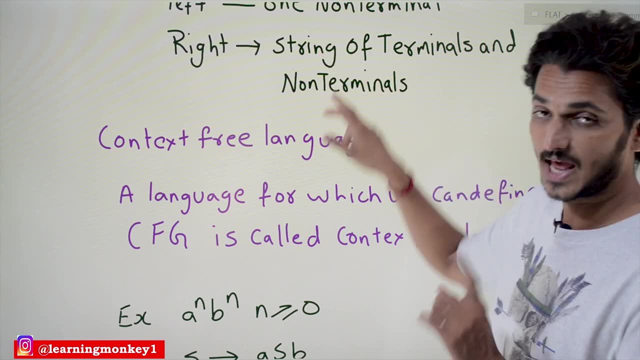 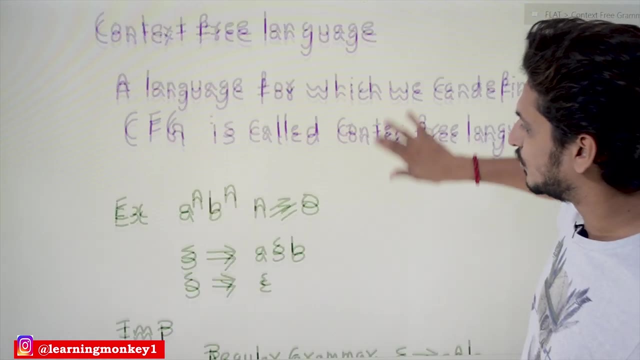 how to write context-free grammar for a given language. that point you will understand in our next classes as of now. these are the conditions to write the productions for context-free grammar, the language that accepts the context-free grammar, for which we can write context-free grammar. we call it as context-free language and, the most important point you have to understand, 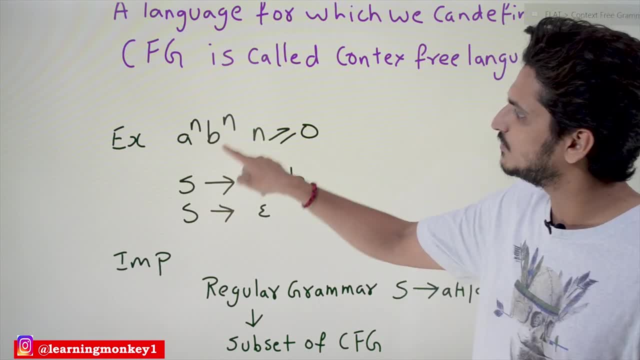 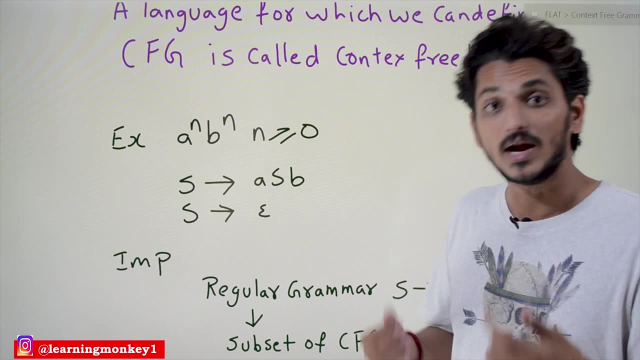 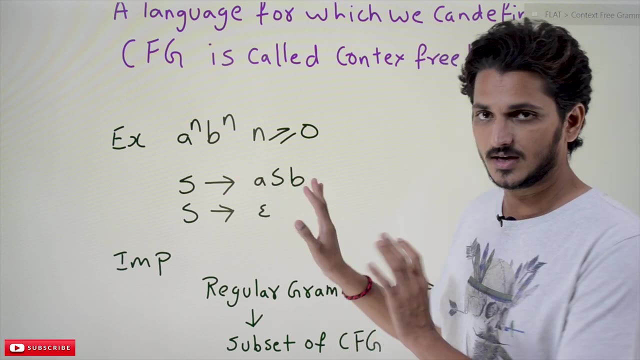 in our previous classes we already discussed that a power n, b power n n greater than or equal to zero. this language is not a regular language. you but we can write grammar for context-free grammar for this language, for example. understand the grammar. how to write this grammar we will understand in our next classes. s tends to a, s, b. 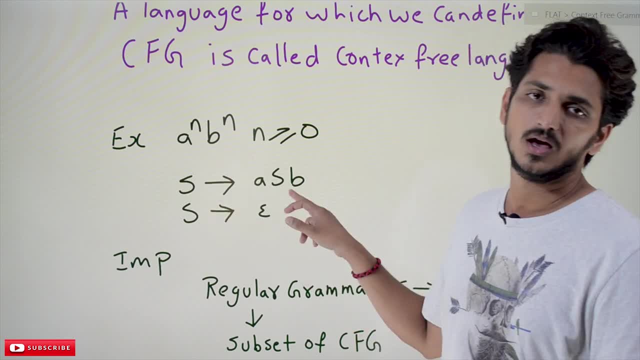 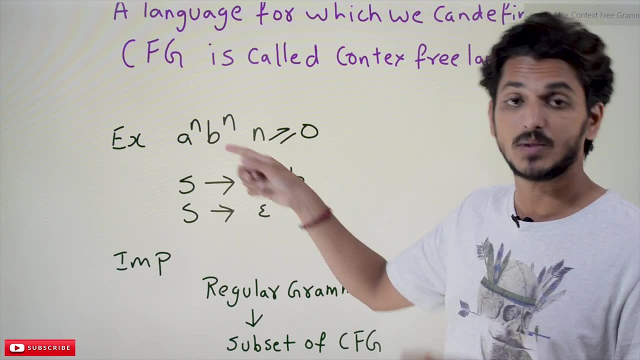 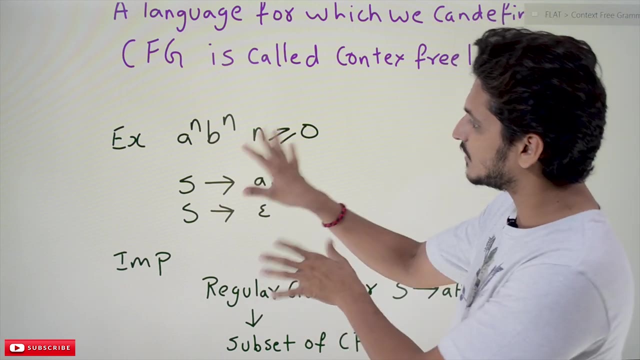 s tends to epsilon. these are the productions for the language a power n, b power n. so we cannot write a regular grammar for this language, but we can write context-free grammar for this language. that's why this language comes under context-free language. we write the grammar for this we will understand in our next classes. and one more important: 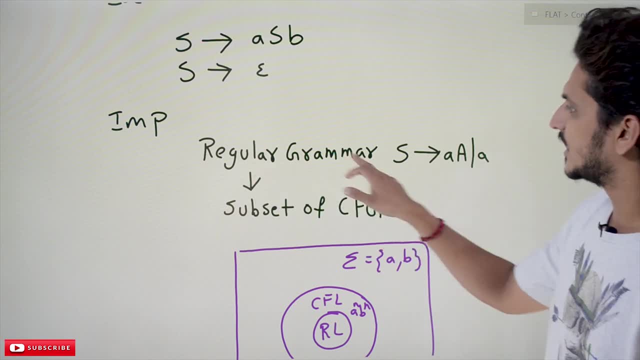 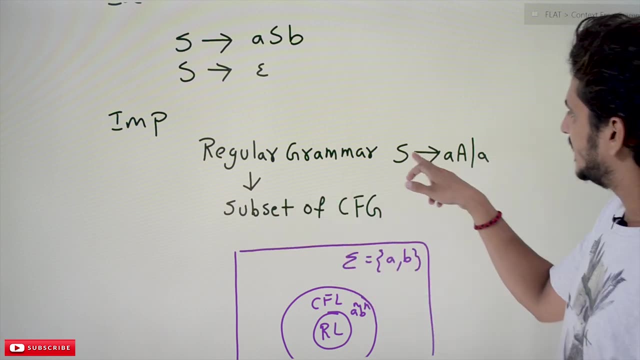 point you have to understand. important point: regular grammar s tends to s, tends to a, s, b, s how the regular grammar will be. it may be right linear grammar, it may be left. linear grammar s tends to a, a or a. we can call it as context free grammar. yes, it is one of the 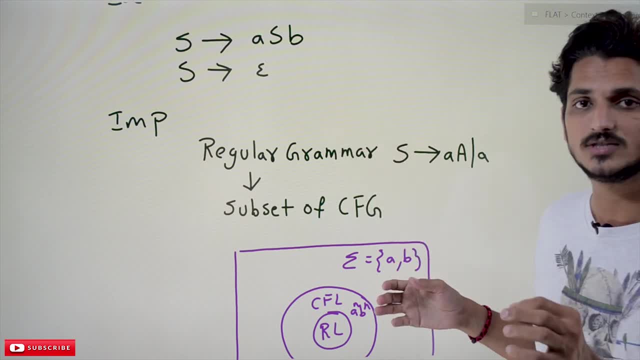 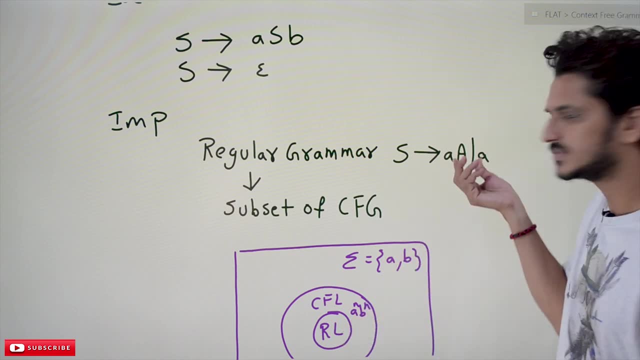 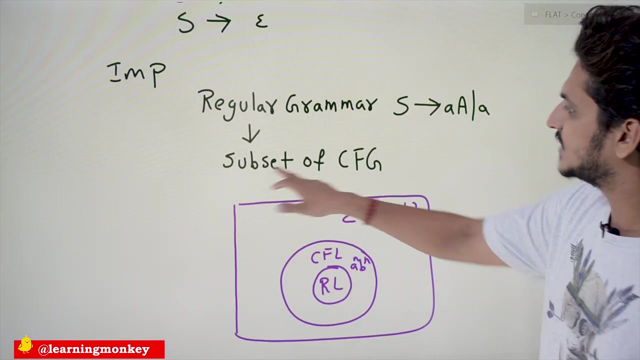 condition in context-free grammar. what is the condition of context free grammar? left side, you should have only non-terminal. on the right side, you can have any sequence of terminals and non terminals. this comes under one of the situation in context free grammar. with this point, you what you have to understand is a subset of cfg. regular grammar is a subset of cfg. 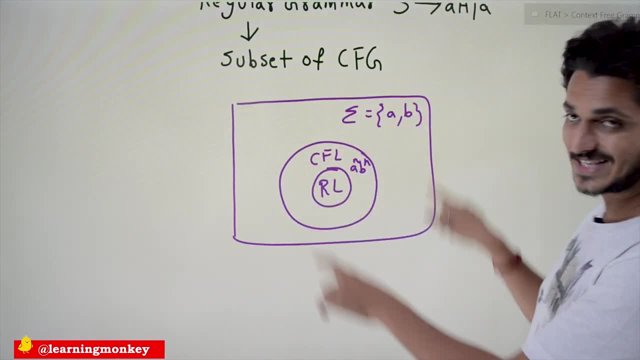 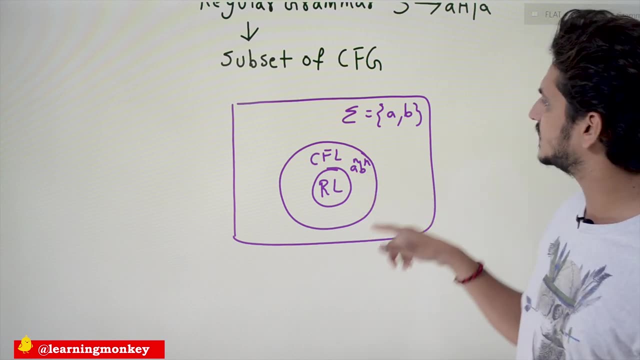 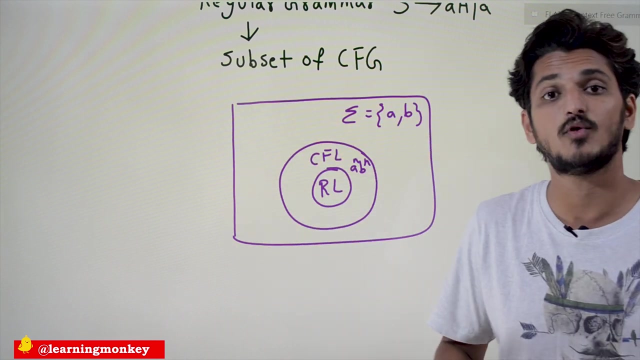 now the point you have to understand is: let's- this is the example which we already discussed in our previous classes- also for regular grammar and regular languages. now coming to the context: free languages sigma is equal to a comma b. this set of, in this whole rectangle, consists of: set of: 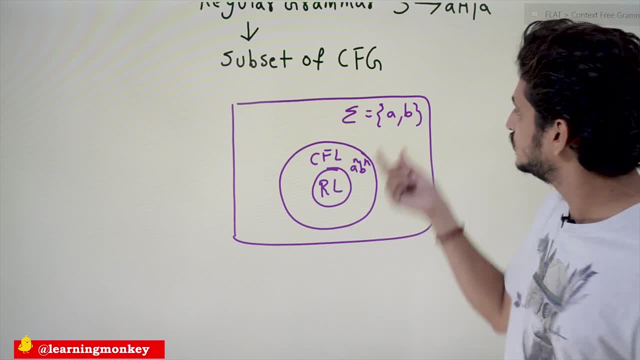 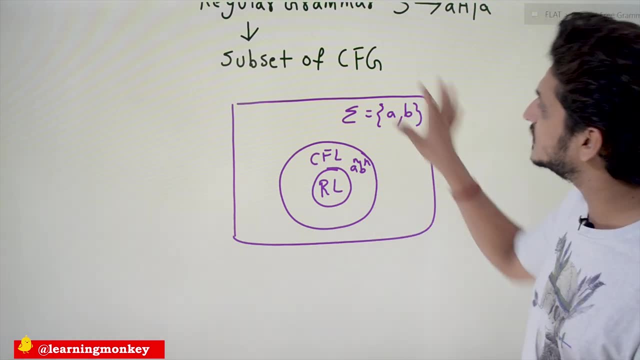 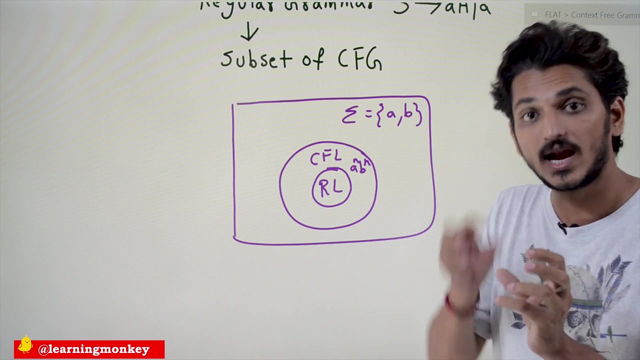 all the languages that we can define using this alphabet: a, comma, b. we can define infinite number of languages out of this infinite number of languages by using regular grammar, we can define only few languages. that languages we call it as regular languages. one of the example which we 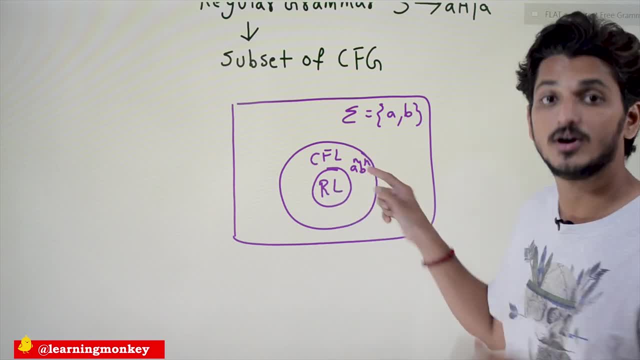 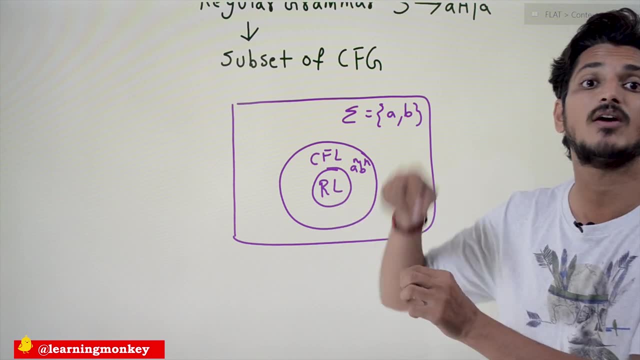 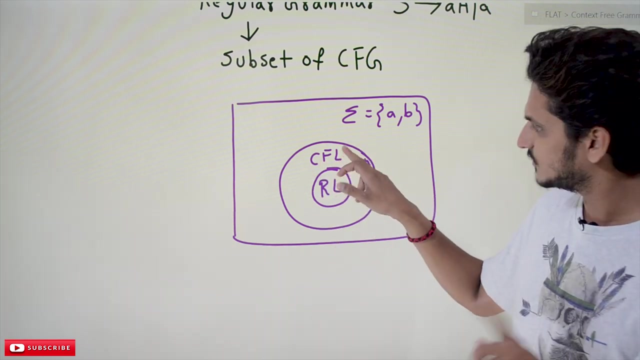 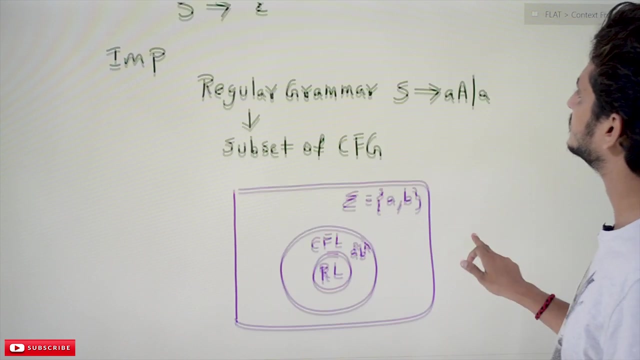 cannot define regular grammar is a power n, b power n for that we can define context free grammar. so for context free grammar, regular languages is a subset of context grammar. then the point is, if you write a context free language, context free grammar can automatically define regular languages also. 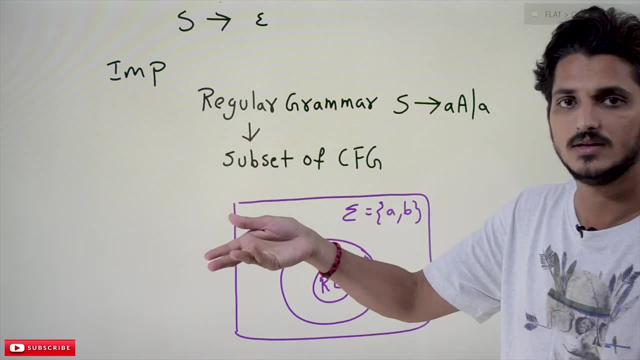 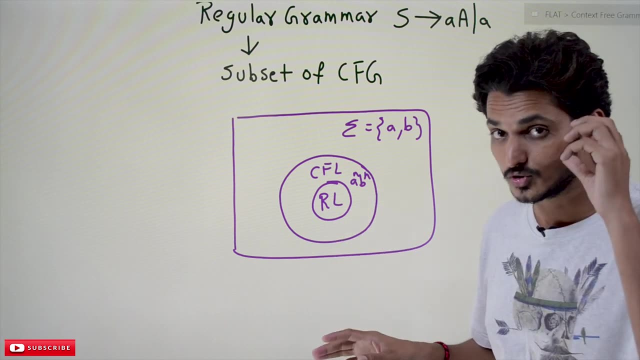 because this is the condition to write the regular grammar. this is one of the condition in context salary grammar. that's why regular languages are subset of context free languages. this is the point you have to understand In order to solve gate bits and many other things. these points are very, very important. 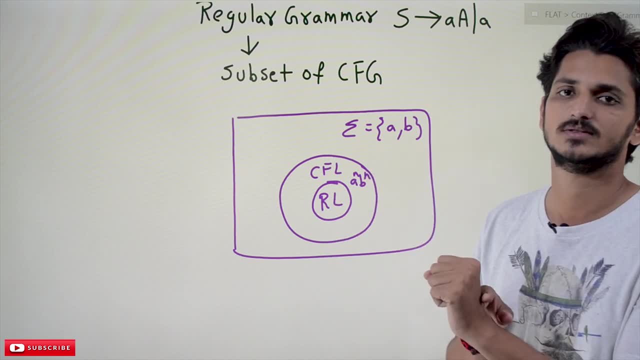 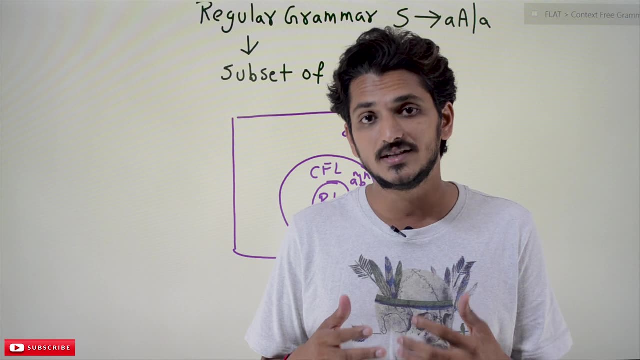 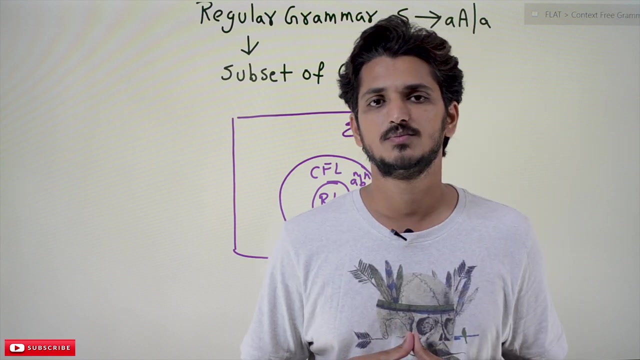 Regular languages are subset of context free languages. Hope you understand about context free grammar and context free language. In our next class we are going to discuss how to write the context free grammar for a given language. If you have any questions regarding the concept, please post your questions in the comment section below. 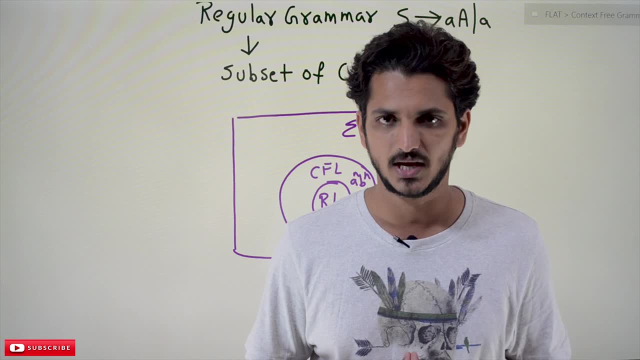 Thanks for watching. If you haven't subscribed to our channel, please subscribe to our channel and press bell icon for the latest updates. Thank you.